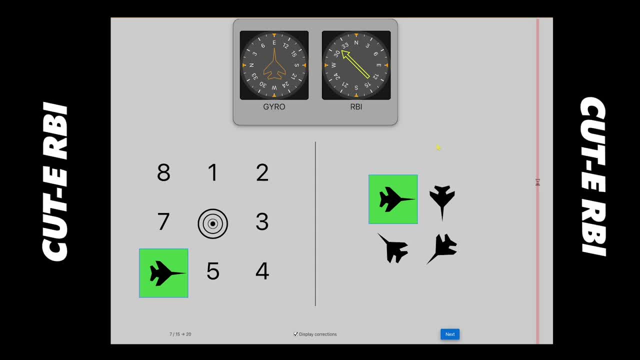 All right, so this is the QT. QT, cut E, however you want to pronounce it. This is the RBI brain game. At first, when I was doing it, honestly, I had no idea what I was specifically supposed to be doing. NDBs- I haven't actually ever flown an NDB, So for all those who haven't, 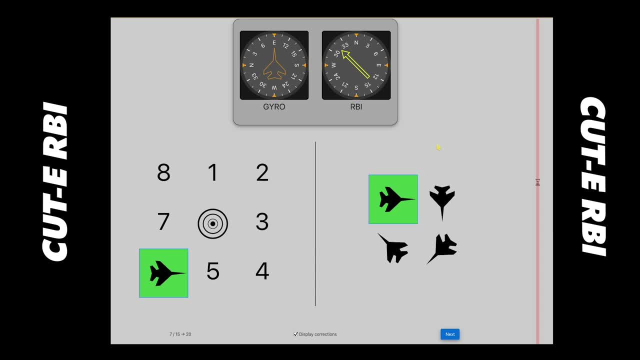 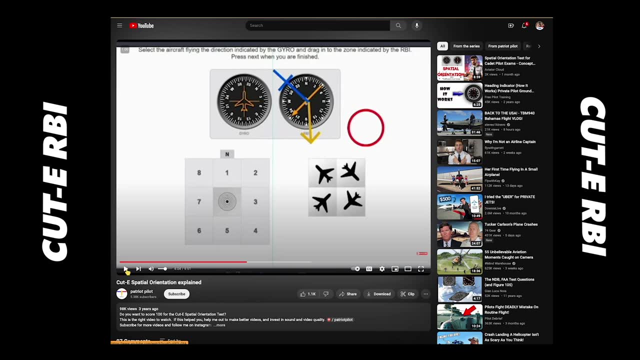 also had that experience. here's how I was able to figure it out. So, basically, this guy's got a really nice start, but it's overly complicated. I ended up figuring it out quite easily that you don't have to draw this little blue line and you don't have to have the yellow arrow. You don't. 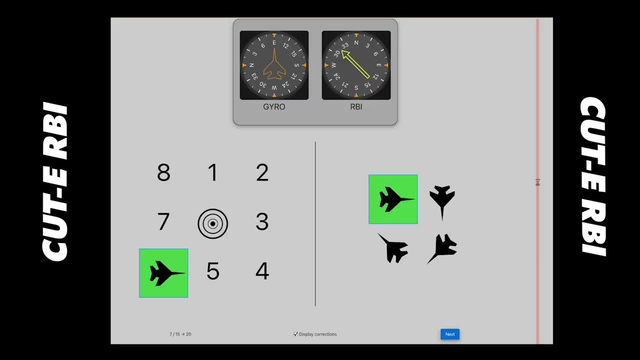 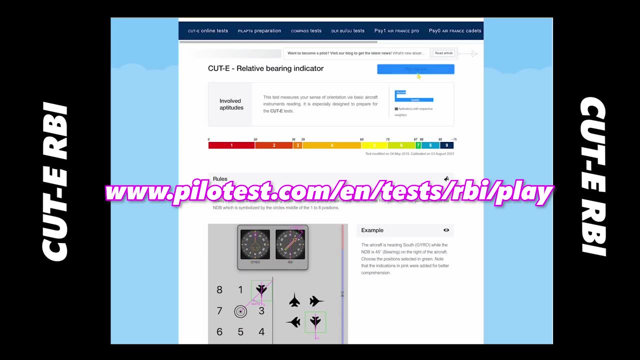 have to any of that stuff. This is how you do it. Again, this is on the cut E pilot testcom slash English test slash RBI. When you sign up and then click play the test. this is what you got going on. So basically, before we skip to the next one, so I can show you in practice, 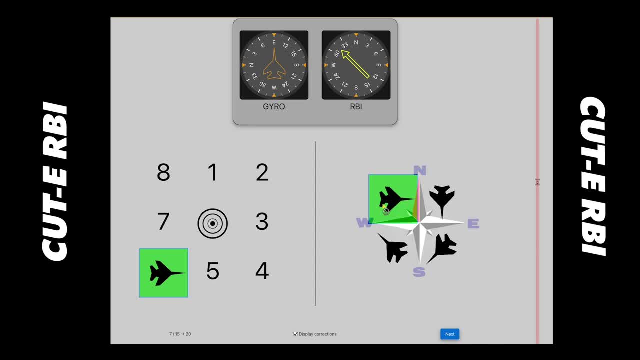 right now the gyro. we are headed east, So pick the bird that is pointed in that direction. That part's really simple. All you have to do is visually cut out this arrow and bring it over to the center of the gyro and have it just point at where that is. So right now it's basically. 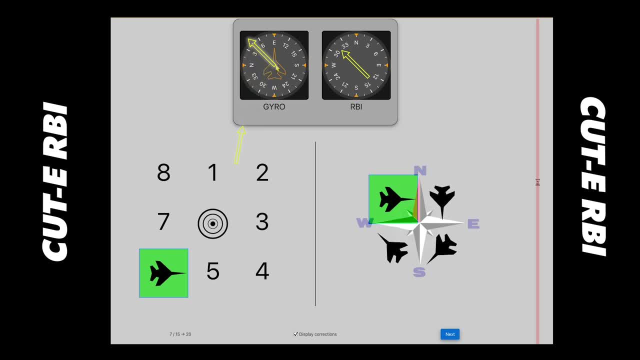 pointing at 045, right there degrees. That's basically what's going to be the bearing to the point. Super simple, Just visually, take this, stick it right in the dead center. wherever that's pointed, that's pointed towards there. So again, if it was like 235, we'd be up here pointing at the at the station, If it was south. 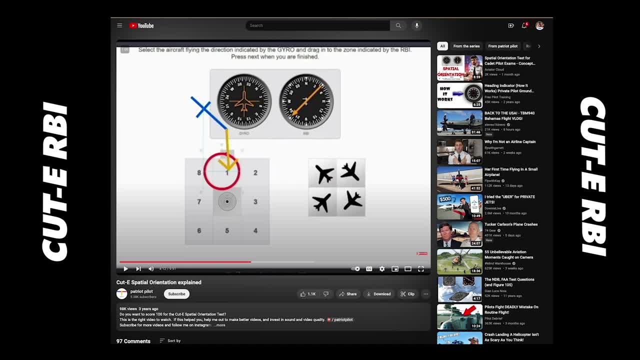 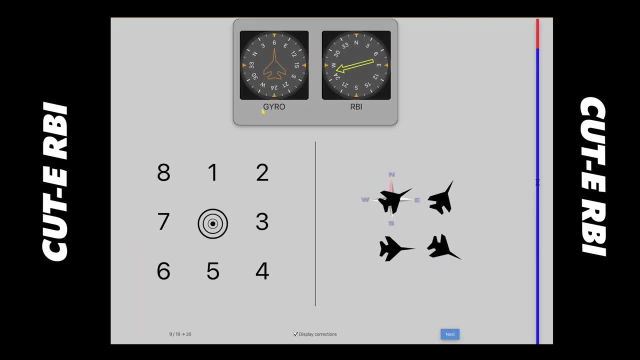 we'd be pointing from one. It's the same thing that he explains in the video over here, where you put it on here and then you rotate the whole thing, but you don't have enough time. This bar is going down, All right, So we are headed to the northeast. There we go. It's actually this one. 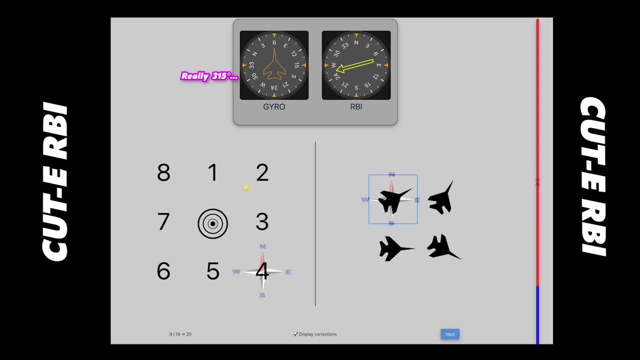 And then we're going to be right there at three zero zero So we're going to go over here. So I want to screwed up because I had the right one going, but really that was, Oh cause it. sorry, I should have put it right at the center. I was looking over here So I was thinking it was. 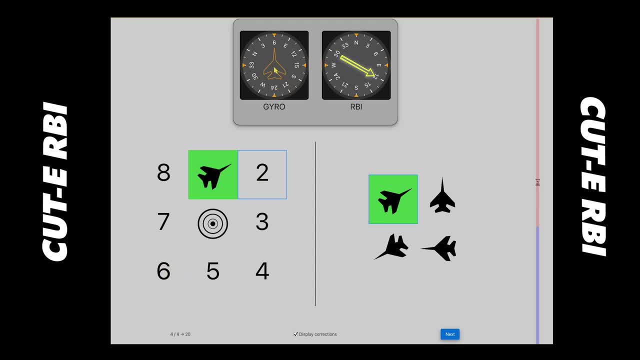 a little bit more off to the edge, but that was: if we draw that line straight from the dead center over, that's that same path. So that's the same path. So that's the same path, So that's the same path. So that's where I screwed that one up. All right, We're going to the south east, and then we 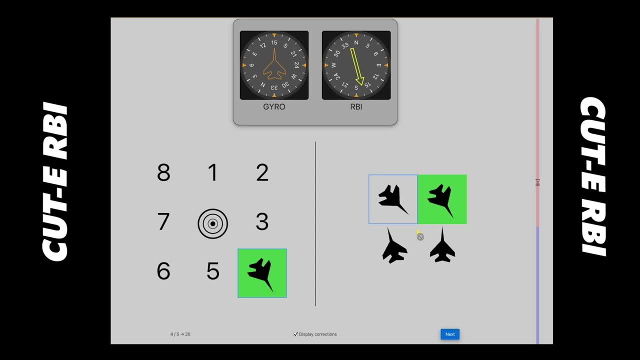 just take that and we're going to the northwest. Oops, That's the slight difference, right? Is that just nibbles off? I should have just looked at it closer that I had that much. So I have to slow down a little bit there. All right South to the southwest, There's only one definitely going down. 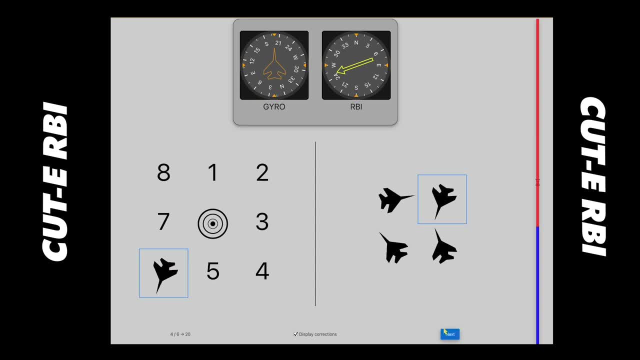 that way And then that's pointed, basically almost a little bit due east, but it's a little bit up there. So that's, is that due east? I got to do a better job. See, look at this, I got to come. 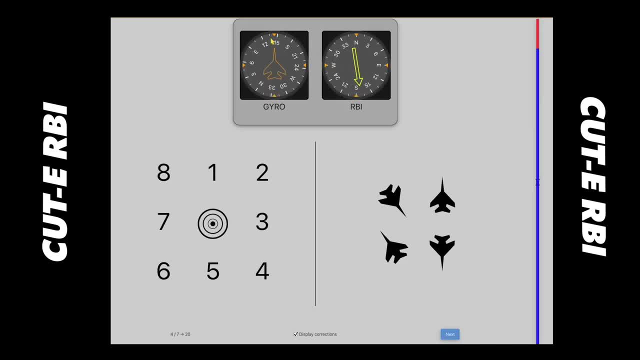 straight from the center. All right, Continue. So we're going to southeast again. We only have one southeaster, and this time I'm going to take it straight off the center, And now that one should be this one. Okay, good, Now we're going just a little bit southeast, not a strong southeast. 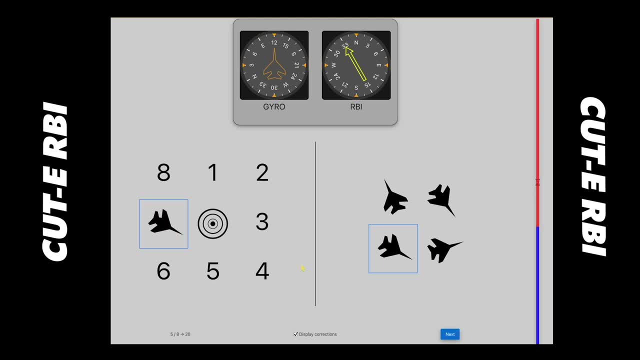 So there's two southeast and then we're taking that back over and that's going basically due east, So that's going to be seven. All right, We're getting it, We're getting it. So that's just a little bit northwest slightly And 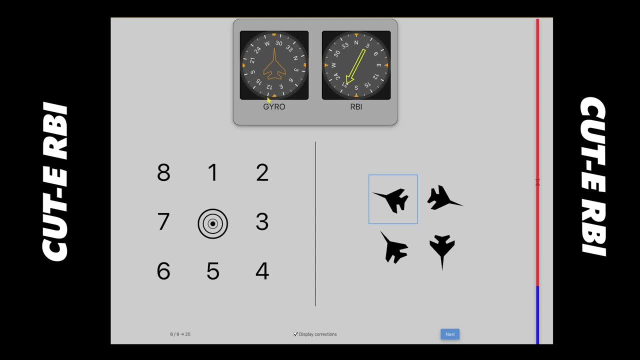 then that's coming over here and we're taking that right about to the oh God, what is that? That's right here. I was going to go click eight. My brain was having a hard time spinning that one around. All right, We're heading to the northwest again. I've only got one northwest. Take that.